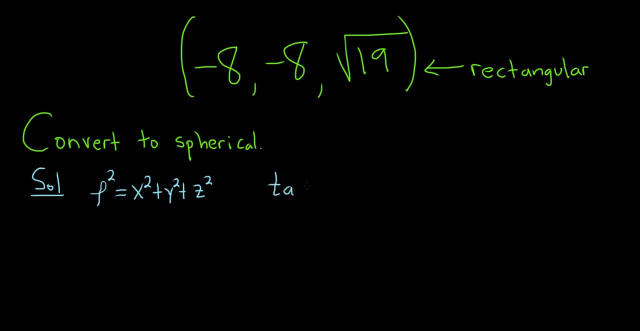 Then we have that the tangent of theta is equal to y over x, And last we have that phi is equal to the arc cosine of, and then it's z all divided by the square root of x squared plus y squared plus z squared. 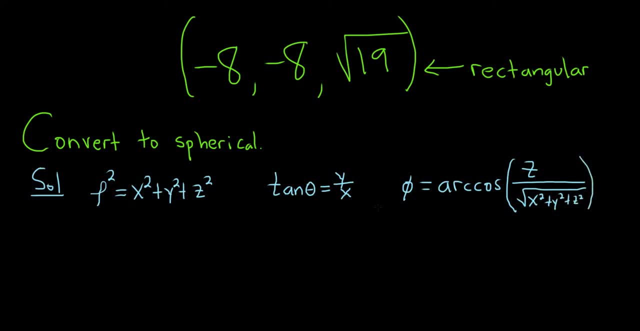 You'll notice that the denominator of this expression is just rho, So books just typically tend to write it this way, with the x and the y and the z, so you can kind of see exactly what goes in there. Okay, and we're given this in rectangular, so we already know our x, our y and our z. 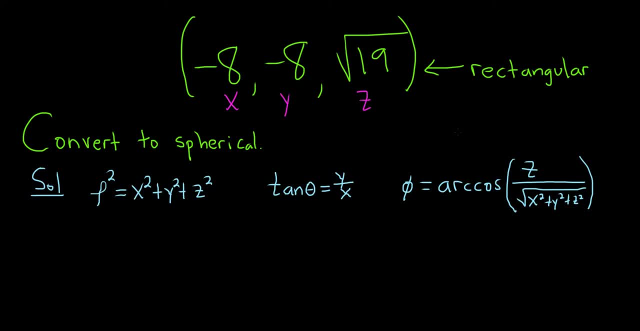 The final answer, by the way, should have the form rho theta phi. Alright, that's the form of a point in a spherical coordinate. so rho theta phi. So rho is equal to the square root of. so we're just going. 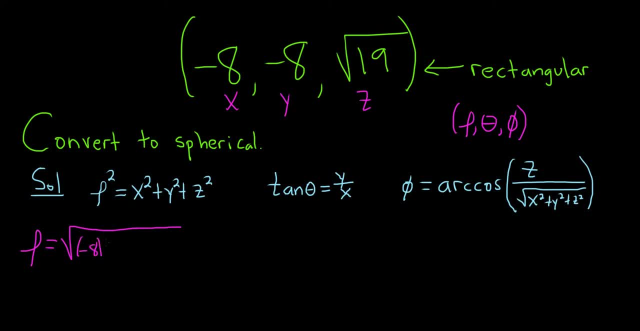 to square each piece here. so negative 8 squared plus negative 8 squared plus, and then the square root of 19.. Quantotom equal to six. Okay, squared. so this will be the square root of so 64 plus 64 plus 19, so Rho is equal. 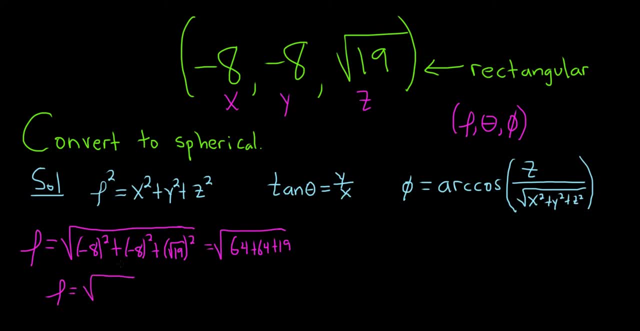 to the square root of. so if you put this in your calculator or you add it up in your head, I'm getting 147. so oftentimes when you get this you try to simplify it. you know, if you can't do it it's no big deal. I believe this is 49 times 3 and so 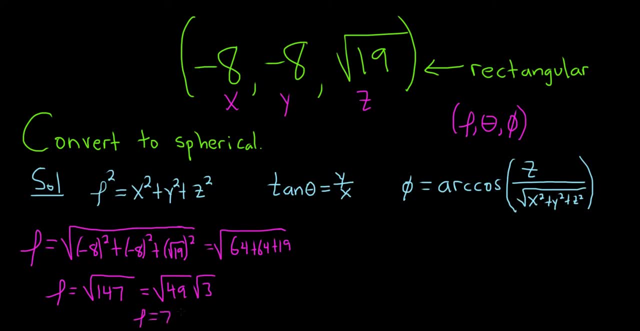 the square root of 49 is 7. so this is 7 square root of 3. so we have Rho to figure out the tangent of theta. the first thing we should always try to do, at least, is use the formula: so it's y over X. so it's negative 8 over. 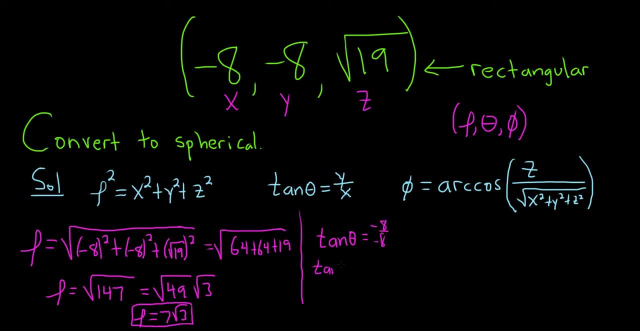 negative 8. so the tangent of theta is 1. so a common mistake here would be people for someone to say, okay, so theta is pi over 4. that would be an incorrect answer, even though theta does satisfy this equation. pi over 4 does work. it is the wrong. 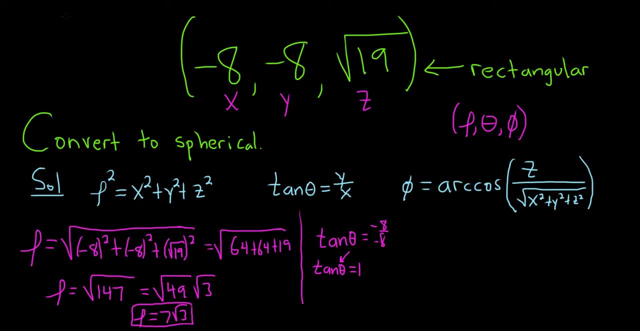 answer. and the reason is: you should always draw a picture when you're doing these problems. so let's draw a picture. there's the y-axis, there's the x-axis and you want to plot your X and your Y in this plane. so negative 8, negative 8 is. 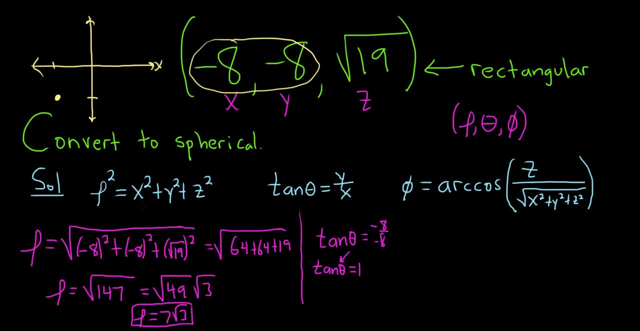 going to be over here- and quadrant 3. so you know, your angle must be a multiple of pi over 4, because the tangent of that angle is 1. and so you say, okay, which multiple is it? well, this is pi, and you can think of pi as 4, pi over 4. so when we're down here in quadrant, 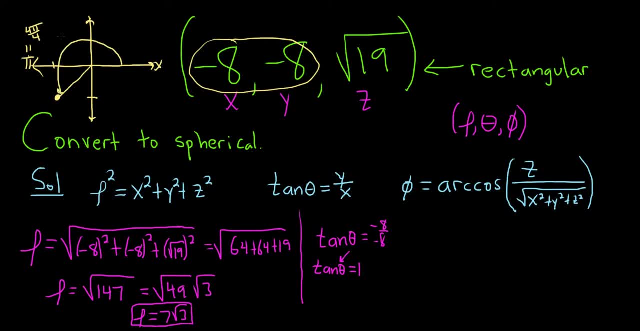 3, you're traveling another pi over 4 radians, So this angle is going to be 5 pi over 4.. So the correct answer in this problem is 5 pi over 4, and this is extremely important. It's probably the hardest thing in this problem. so 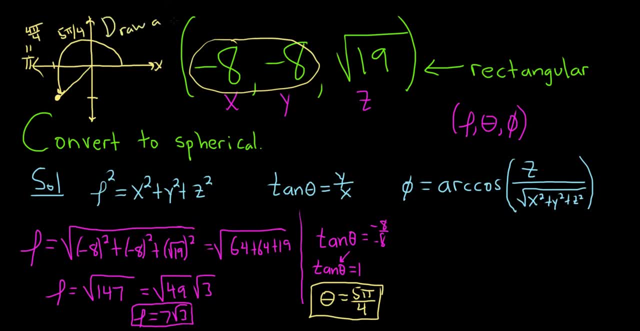 don't forget to draw a pic when you're finding theta very key. The last piece is to find phi. So phi is equal to the arc cosine of z, which is the square root of 19,. over this expression here, But we talked about this. this is just rho. so this is 7 square root of 3.. 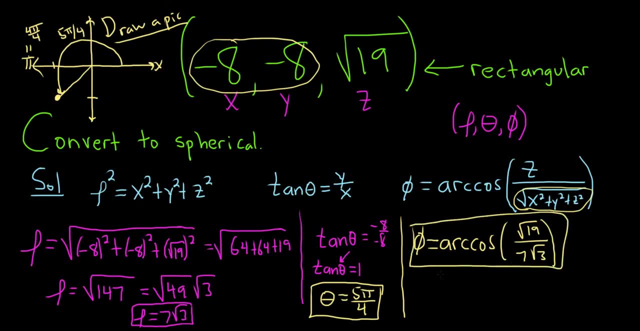 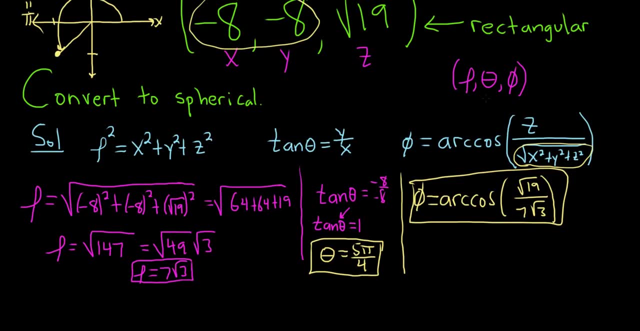 And you can just leave it like that. that's perfectly okay, no problems there. And so now we're done. We're going to have to write our answer in the correct form, So remember the form is rho theta phi, so this will be rho, which is 7 square root of. 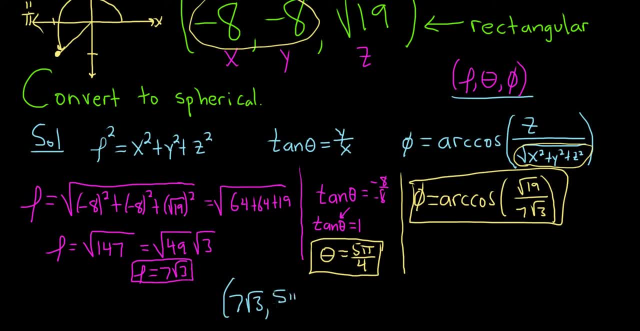 3, theta, which is 5 pi over 4,, and phi, which is the arc cosine of the square root of 19 over 7 times the square root of 3.. What a beautiful number, Beautiful order tree Triple that is.